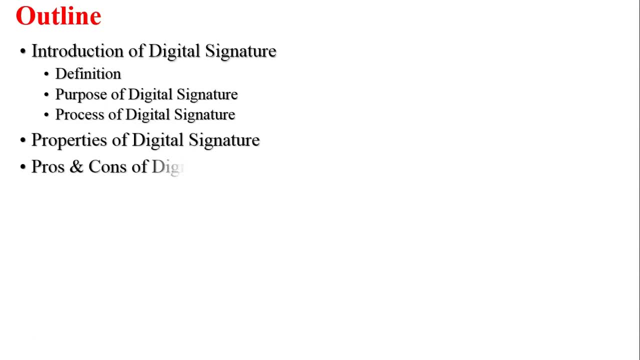 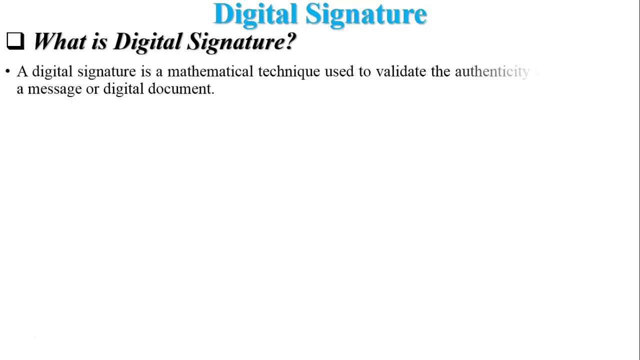 Fourth one: properties of digital signature. Fifth one: pros and cons of the digital signature. So let we discuss with introduction of digital signature, with definition. So first of all, what is digital signature? A digital signature is a mathematical technique used to validate the authenticity and integrity of a message or digital document. Here, two words is most important. One is authentication, or we can say authentication. 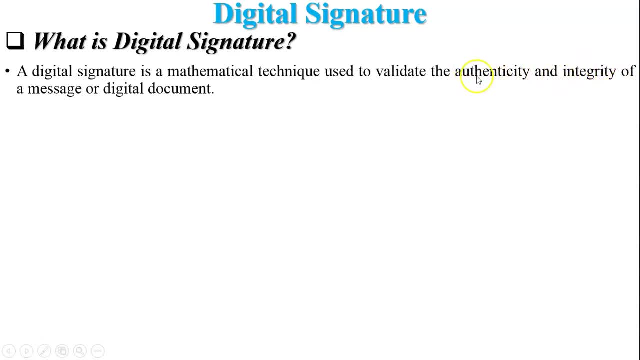 First one is authenticity and second one is integrity. Authenticity means sender must have to prove that this message is sent by valid sender, And integrity means message should not be altered during the transmission of message. Whenever we think about digital signature, there is one image in our mind: like that way The document is signed by digitally, But this is not actually digital signature. Now check the proper definition of digital signature. 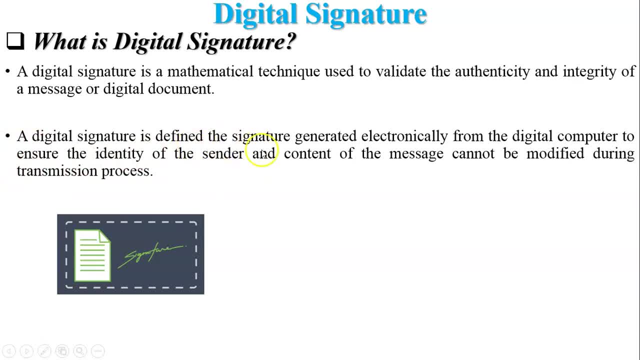 A digital signature is defined, the signature generated electronically from the digital computer to ensure that the identity of the sender and the content of the message cannot be modified during the transmission process. Here, identity of the sender, it means it provide the authentication. and content of the message cannot be modified during the transmission process, It provides the integrity. So this is the original definition, or we can say proper definition, of digital signature. 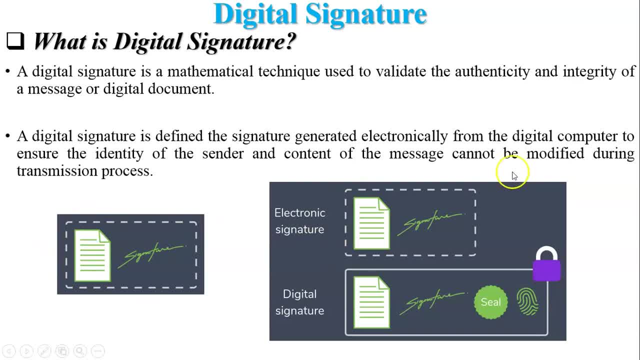 Now see another figure. So this figure is called electronic signature and this is digital signature. Here in this digital signature there are two different marks over here. This is the thumb print, or we can say this is the identity of the sender and this is lock, or we can say it is protected by any of the algorithm. Another one: this is seal. Seal means if anyone wants to modify the message, this seal will be broken. So we can say there is. 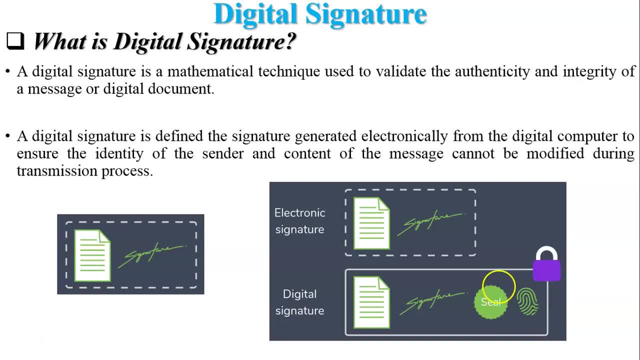 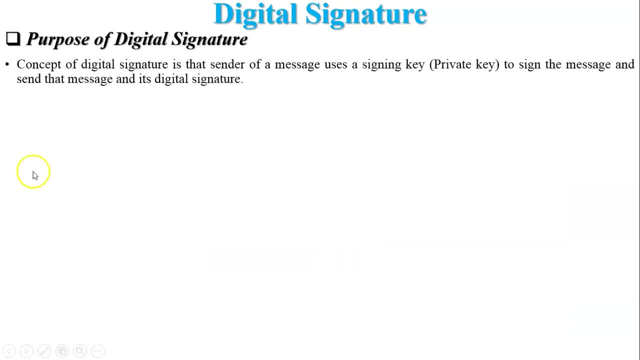 integrity inside the message. if anyone modify the message, this seal or we can say the value of this particular is change. so this is called digital signature. now, purpose of digital signature. the purpose of digital signature is that concept of digital signature is sender of a message uses a signing key, or we can say private key, to sign the message and send the message and its digital 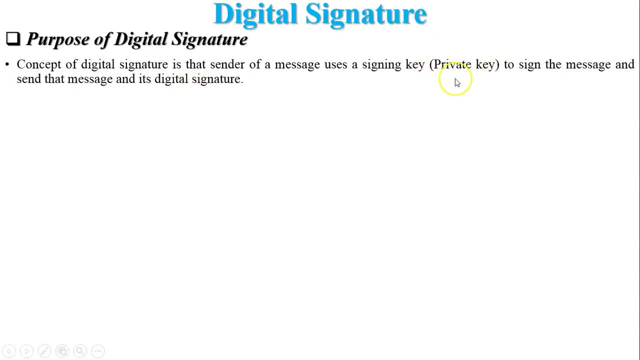 signature: here private keywords is used. it it means digital signature, mostly based on public key cryptography. so it means here sender will sign with the help of this private key and sign the message and send to the receiver. here digital signature and message. both are appended and sent to the receiver. the receiver uses a verification key here. verification key is public key of the. 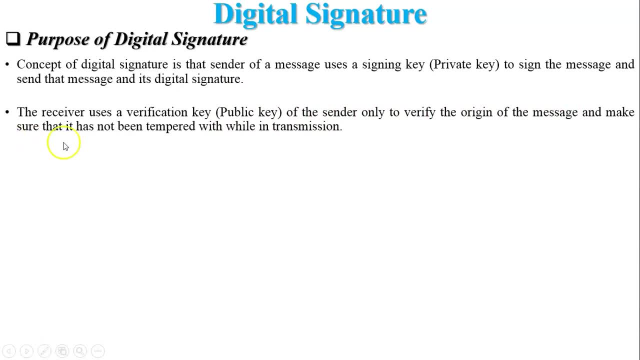 sender only to verify the origin of the message and make sure that it has not been tampered with while in transmission. it means there is no integrity in the message and message will be sent by original sender. it will be checked by the receiver. here public key and private key is used. it means public. 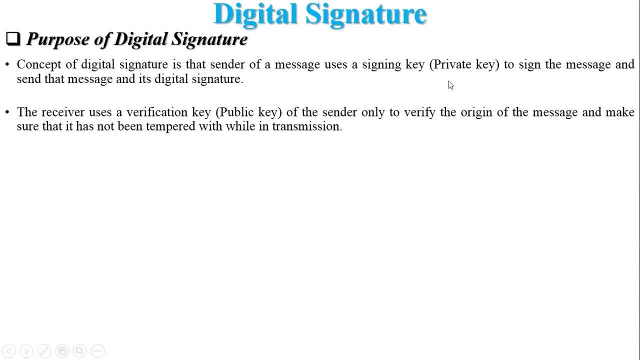 key cryptography is used in the digital signature so we can say if sender will, first of all, sender will generate public key and share with the particular user or all the user connected in network. so digital signature technique achieve the authenticity and integrity of the data or internet. we have already discussed about that. 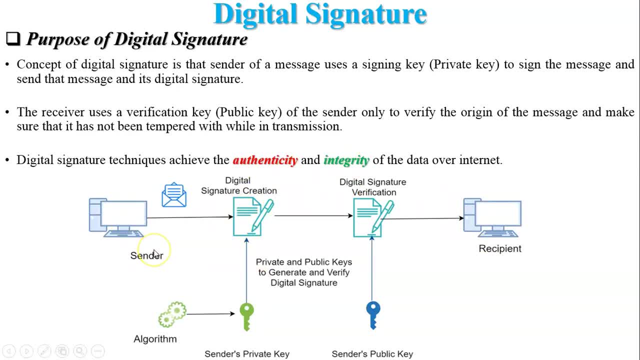 here there is one scenario of digital signature you can see over here. this is the basic diagram of digital signature. this is sender side. this is receiver side. from sender side, message will be signed by digitally. it means message will be encrypted using the private key- private key with the help of some of the function or some of the algorithm and sent. 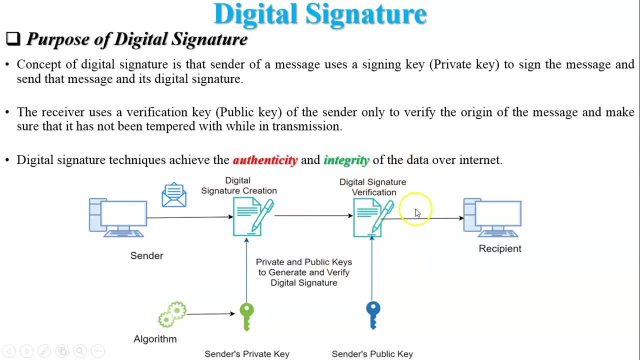 to the receiver side and receiver side receiver will decrypt this message from the public key and check there is no integrity in the message and this message is authenticated. so then, and then receiver will receive the message. now discuss about process of digital signature in detail and step-by-step. 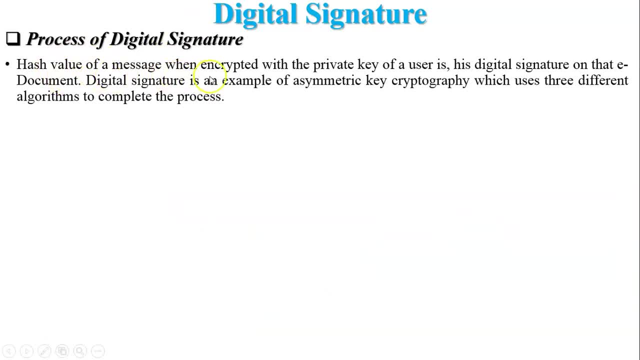 of digital signature. so hash value of the message when encrypted with the private key of a user, is his digital signature on that e-document. so digital signature is an example of asymmetric or public key cryptography which uses three different algorithm to complete this process. first of all, we discuss about this statement, find the hash value of the given message and encrypted with 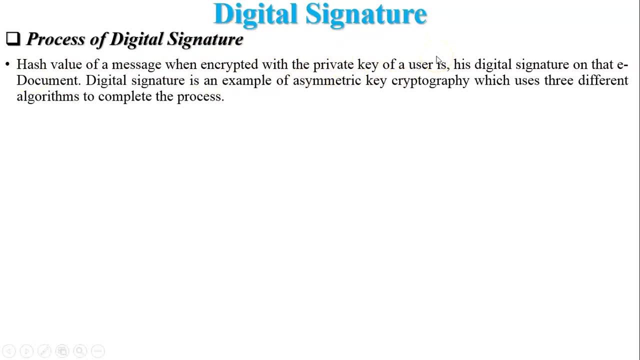 the private key and send to the user, or we can say send to the receiver. it means if anyone wants to change this message, the hash value will be changed and if anyone wants to decrypt that hash value, that person or attacker must have received the public key of the user, or we can say of the 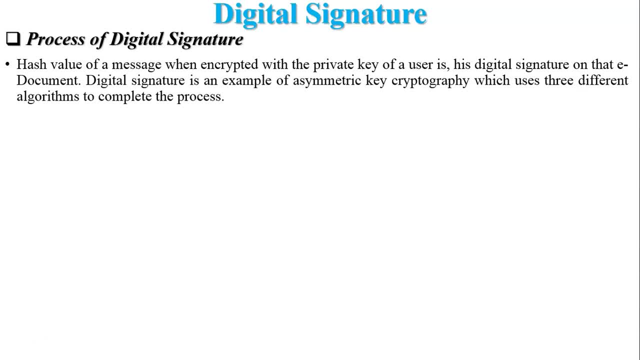 sender now discuss three different algorithm is used for this process. so first, one first step is key generation algorithm, which generates private key and corresponding public key, and public key is shared with the users, which is connected in network by the sender. second algorithm, next step, signing algorithm- is 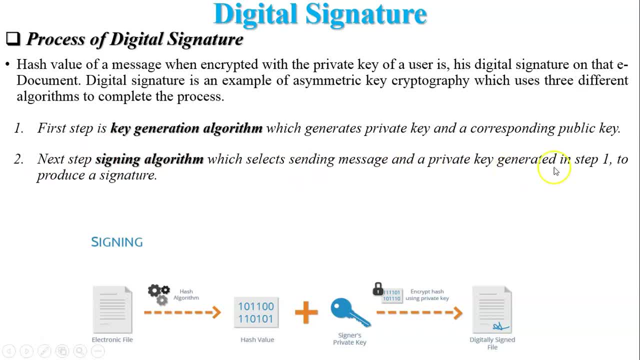 used with select sending message and private key generated in step one to produce a signature. now see in this figure. this figure shows the signing algorithm here. electronic file, we can say our data or mdfi, and generate hash value. hash value is encrypted using the private key. private key is: 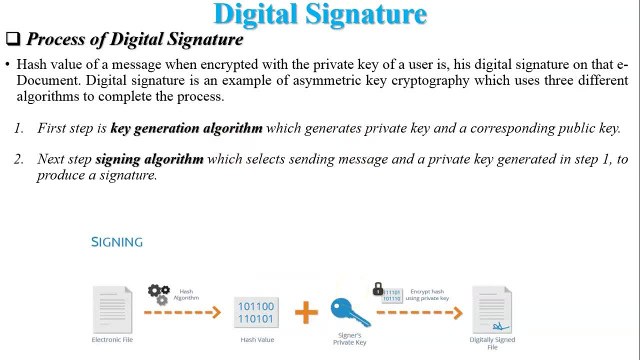 generated from step number one. so this encrypted hash value is attached with that document. now you can see over here: this is encrypted using the private key, this hash value, and attached with document. it means this document is digitally signed or we can say digitally signed file. next third step is verification process. verification process is executed. 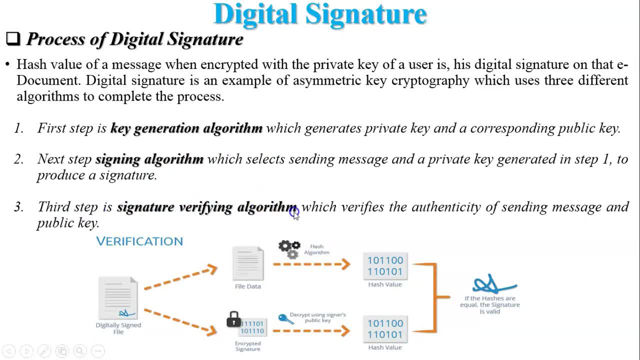 in the receiver side. so third step is signature verification algorithm is used which verify the authenticity of the sending message and public key at the receiver side. in this figure, receiver will receive digital signed file and remove this data file and this encrypted signature, or we can say encrypted hash function from the file. receiver will generate a hash code and decrypt that encrypted 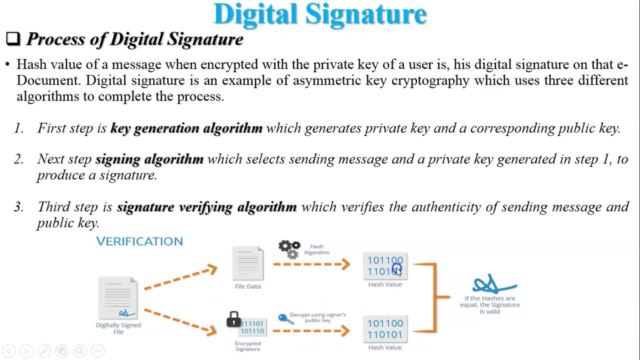 hash code with the help of senders, public key. if both hash value are same, it means signature is valid. or we can say: there is no forgery in the message and message is sent by the originally sender. so this is the verification process. so this is the process of digital signature. both figure are combined for the signing and 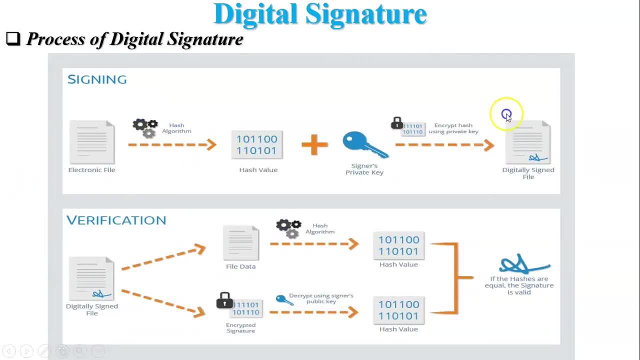 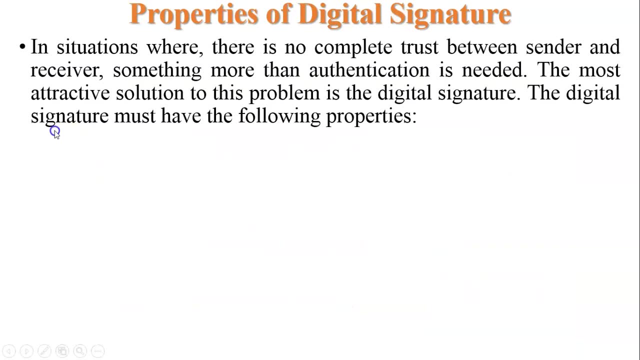 verification: this is the signing and this is the verification. so above figure as the sender side and below figure is at the receiver side. now properties of digital signature. in situation where there is no complete trust between the sender and receiver, something more than authentication is needed. at that time digital signature is used, the most attractive solution. 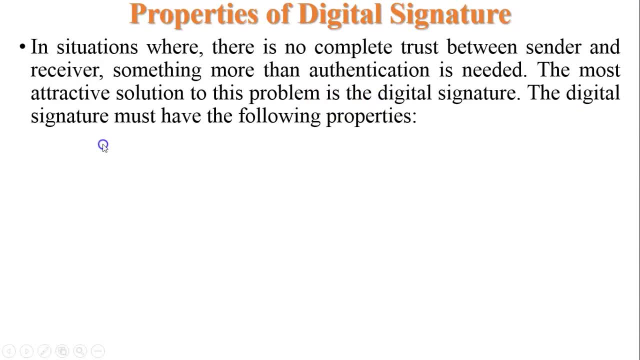 to this problem is the digital signature. the digital signature must have the following properties. so first property of the digital signature is it must verify the author and the date and time of the signature. if there is date and time of the signature is not proper and it means receiver. 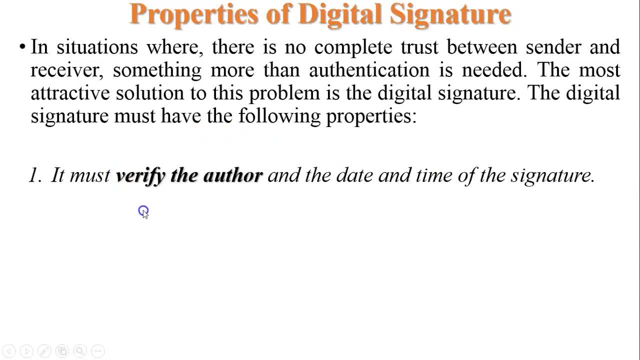 will not accept the message. also, receiver will check the message is sent by the original sender. it means verifiable of the sender or verify of the message author. second one: it must authenticate the content at the time of signature, before doing signature. or we can say before add: 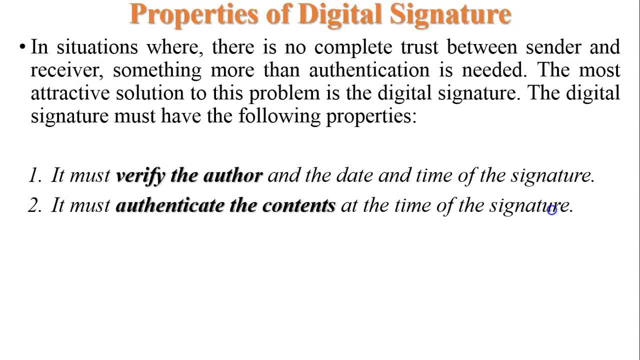 digital signature in the particular file, or we can say in the particular data user, or we can say sender, will authenticate that message. third one: it must be verifiable here: greed also to handle the external messageles means they have to send those messages. there is a benefit to these messages, same ones you can panic out with you For using. how to delete is wait the time This video will be before doing signature, or we can say before at digital signature in the particular file. or we can say in the particular data: user: Ven judicial results will authenticate the message did indeed. 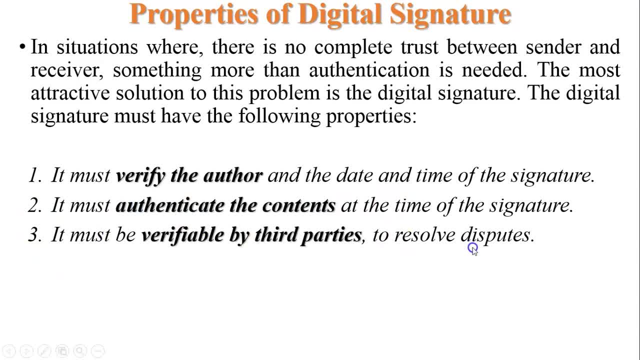 can automatically send it or can also use the captions搶 full type out. can automatically edit the message. it must be verifiable by the third parties to resolve that dispute. it means sender and receiver have no trust at that time. third party will be in picture and verify the digital. 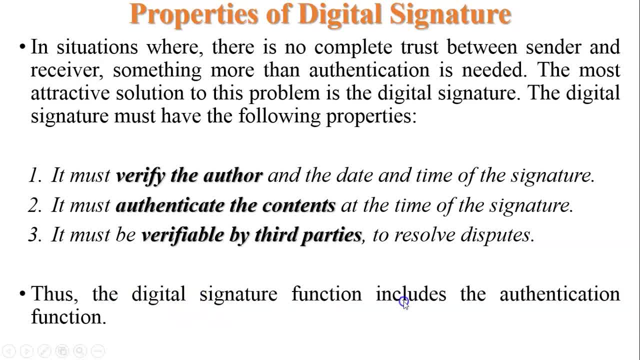 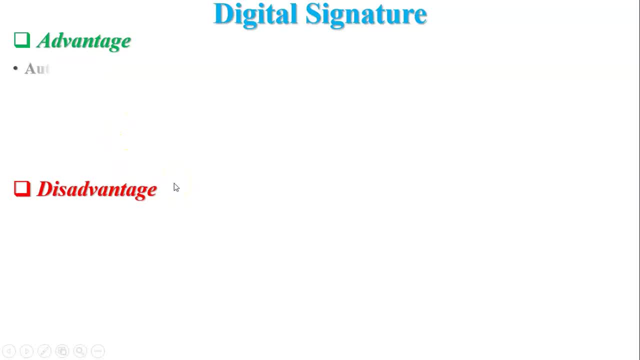 signature. thus the digital signature function includes the authentication function. next, advantage and disadvantage of the digital signature. first advantage: authentication. authentication means identification of the person that sign. second one: integrity of data. every change will be detected because hash function is used in the digital signature. if there is any change in the message, so property of s function has value, will be changed. 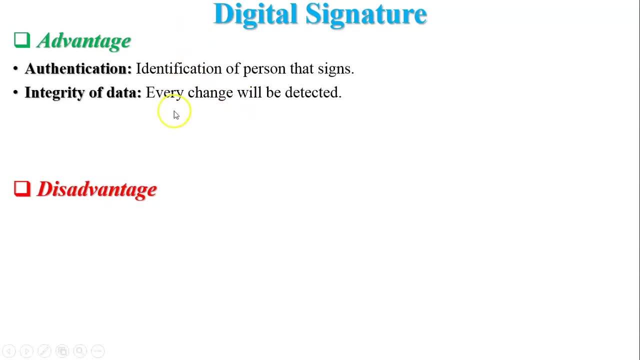 so we can identify the integrity of the data and authentication. third one: non-repudiation. author cannot be denied of his work. if any author will create digital signature and send to the receiver, then author, or we can say sender, cannot deny that work. fourth one: imposter.